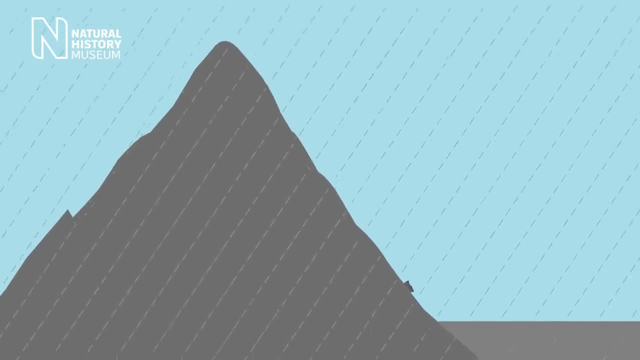 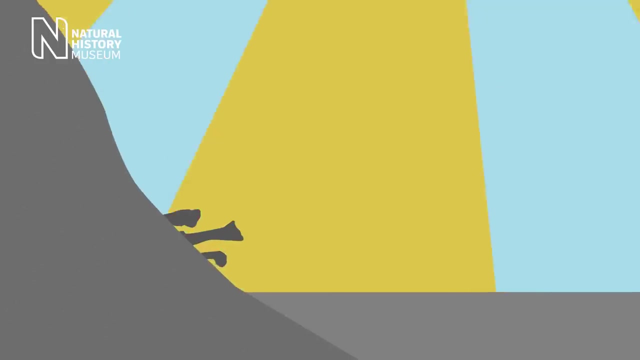 Very slowly. wind, water and ice wore away the rock. Eventually, bits of the fossil skeleton were exposed and became visible on the surface. Fossils are constantly getting eroded out of rock. Most are lost, But if we're lucky, someone will find one. Nearly all of the fossils we find- around 99%- are from marine animals such as shellfish and sharks. This is because they lived in the sea, where sand or mud could bury their remains quickly after they died. But dinosaurs live on land, So how do they get buried so quickly? 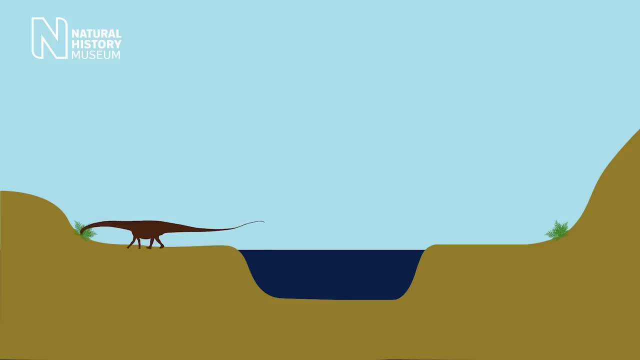 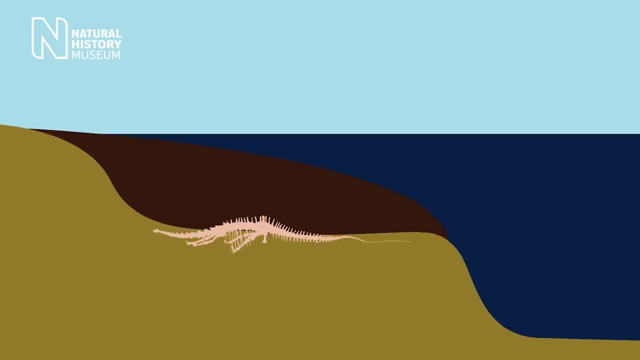 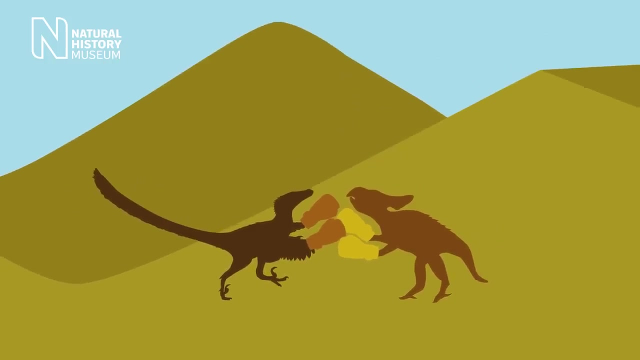 Most dinosaur fossils we find belong to animals that were living near to a lake or a river. They died and a short while later the area flooded, covering their remains in mud and silt. Occasionally, something more dramatic happened. In one example, two dinosaurs, Protoceratops and Velociraptor, were fighting in the desert. 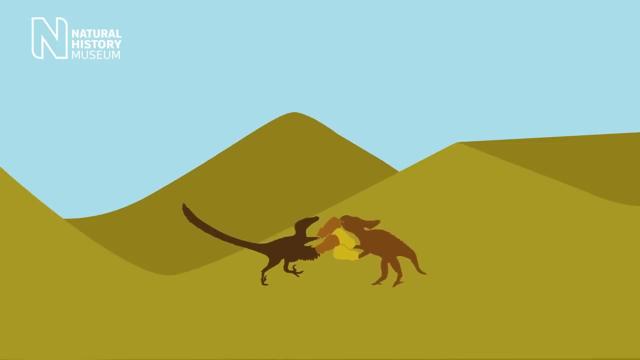 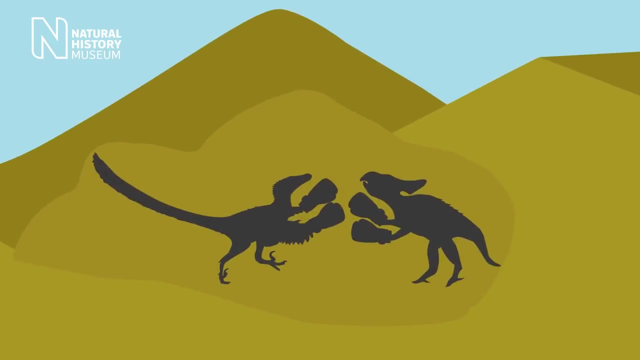 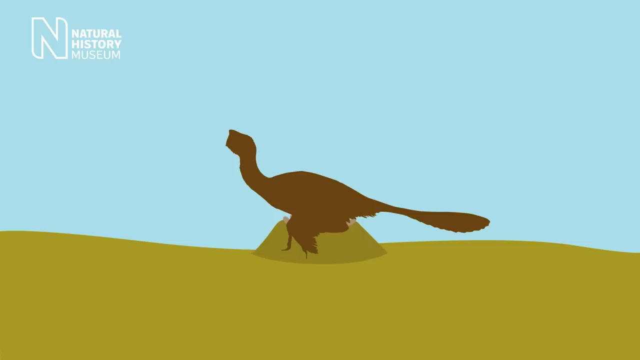 They were mid-battle when suddenly a sand dune collapsed on top of them. Their fossils show them frozen in their fighting poses. In another tragic example, the feathered dinosaur Sitypati was sitting on its nest of eggs when a sandstorm blew in and covered it. 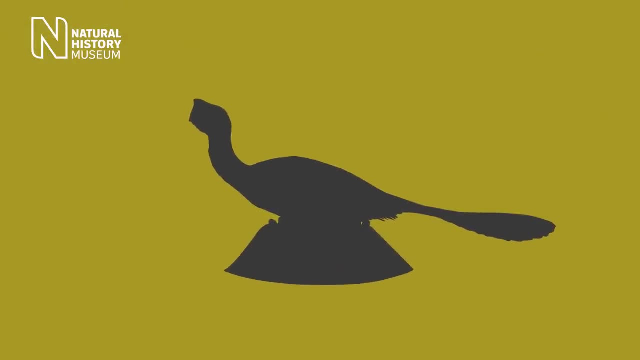 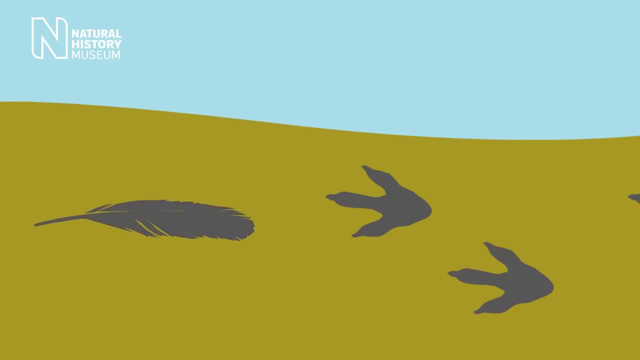 Fossils like this from animals that were alive when they were buried are really rare. It's not just bones that turn into fossils: Dinosaurs can also leave behind footprints and impressions of skin and feathers. So next time you're near some sandstone or mudstone, think of what fossils could be hiding. 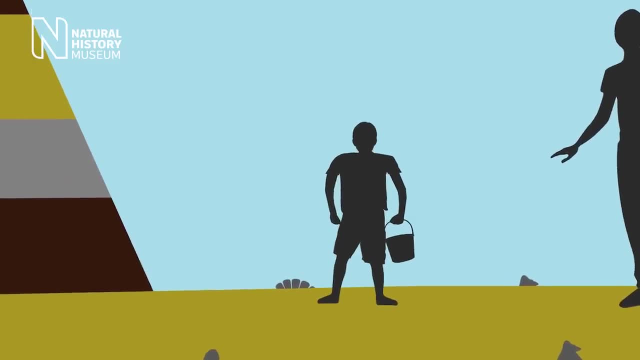 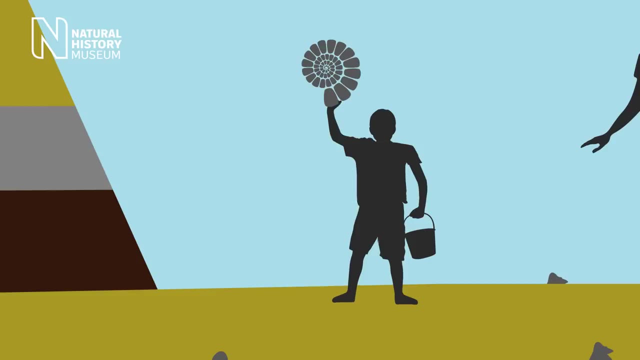 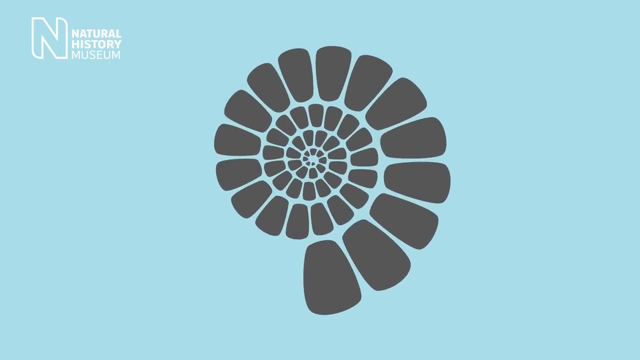 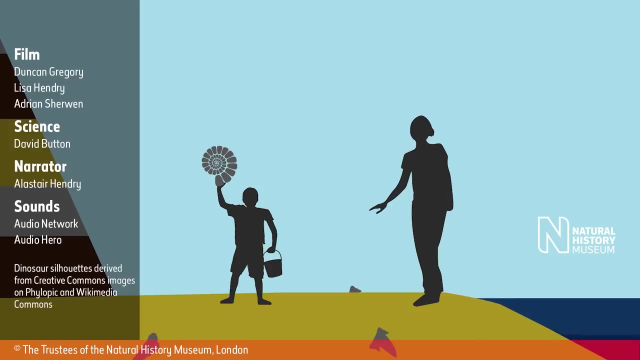 Just waiting to be discovered. It probably won't be a dinosaur fossil, as they're so rare, But it could be a prehistoric sea creature, like an ammonite, which went extinct at the same time as dinosaurs many millions of years ago, Or probably a dinosaur that appeared in the desert. That's only a theory, But it could be a dinosaur that appeared in the desert or, like a dinosaur from the desert, that came from a desert. It's possible that it's a dinosaur, a dinosaur from the desert, but it's a dinosaur from the desert. or it might be a dinosaur from the desert.